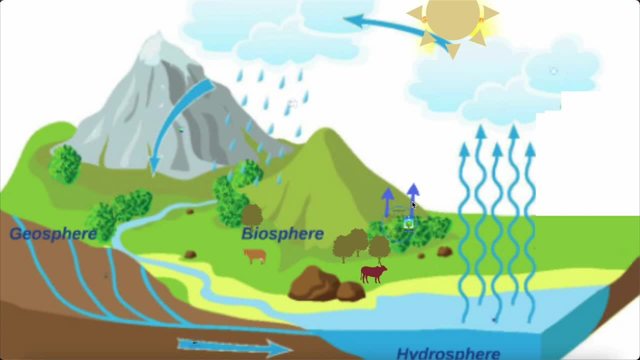 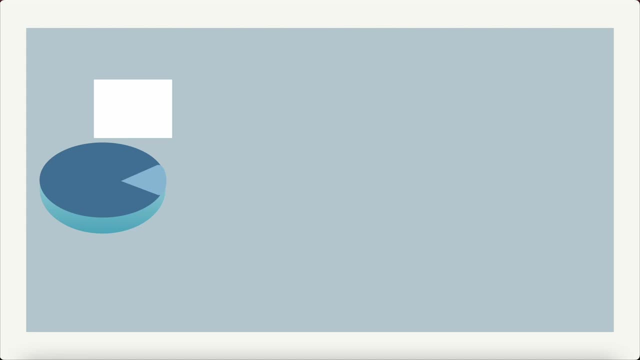 Eventually, the water vapor is given off to the atmosphere. That process is called transpiration. So, moving on to the next slide, how is water distributed? Most of the water in the Hydrosphere- roughly 97% of it, is the salt water, That's, the oceans. Only 3% is the freshwater. as we 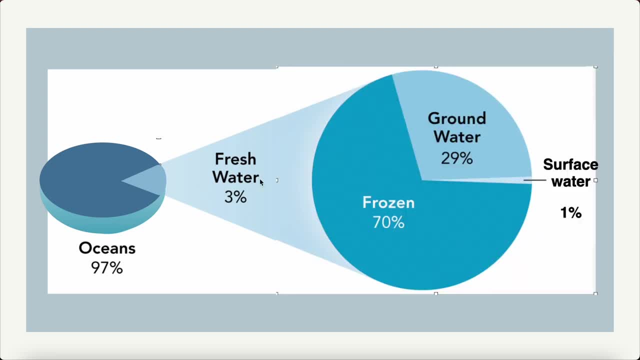 see in here, That's a really small amount. Yes, And in that, the 3% of the freshwater, most of it would be the frozen water. Almost 70% of it is the frozen water. Much of the Earth's freshwater is frozen into the ocean. Yes, When we do that, we demonstrate how much 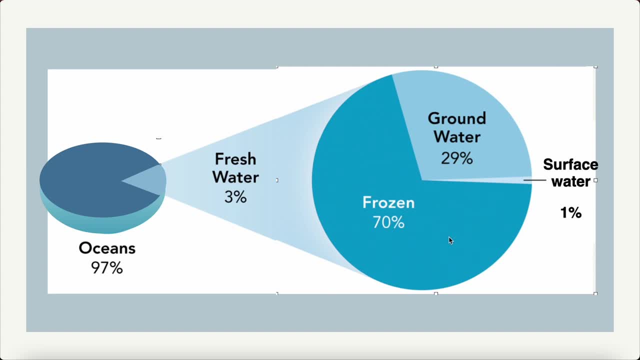 water is solid. At the same time, the water will evaporate and evaporate, Yes, In the into thickened ice masses called glaciers, massive glacial ice sheets cover most of the greenlands and antarctica. about third of earth's fresh water is the groundwater, underground water- a tiny. 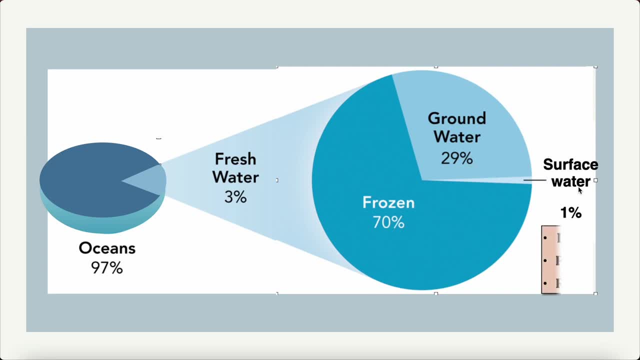 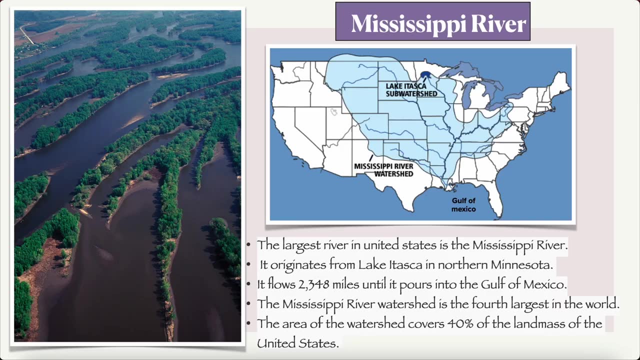 fraction of fresh water occurs in the form of surface water. that would be the lakes, ponds and rivers. so, now that we saw the lakes, ponds and the rivers, where the tiny small amount of surface water, let's start with river which is the largest river in united states. it's the mississippi river. 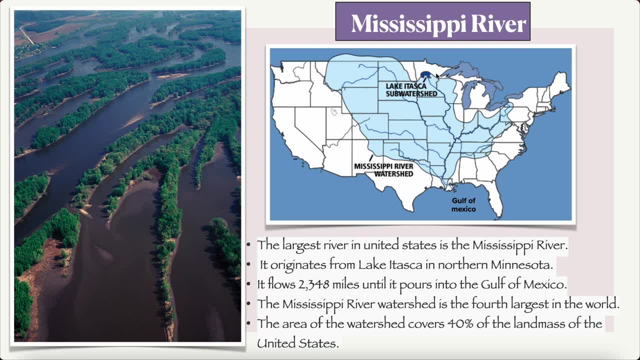 and it originates from a lake called itasca in the northern minnesota. it flows to 1348 miles until it pours in gulf of mexico. that's where it ends. the mississippi river's wash shed is the fourth largest in the world. the area of wash shed covers 40 percent of landmass of the united state. 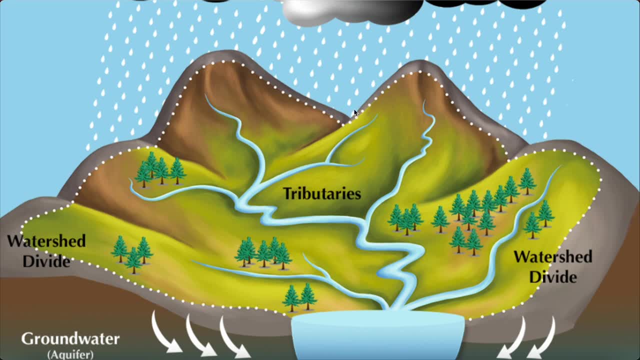 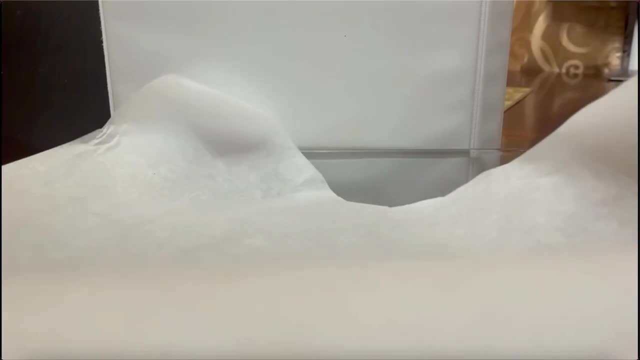 so what is the largest river in the united states? what does wash shed mean? this entire area that you see is a wash shed. how? how watershed works. yes, here i've got a parchment paper which i'm crumpling it up into a ball and then i'm spreading. 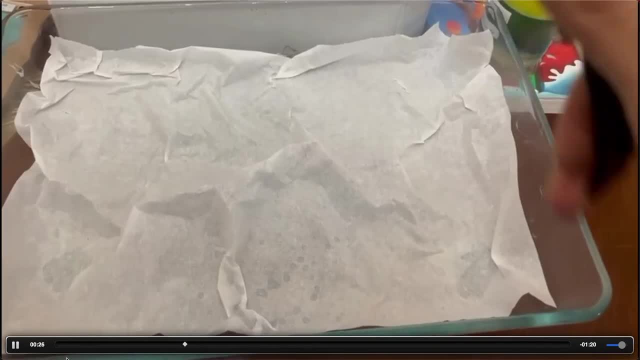 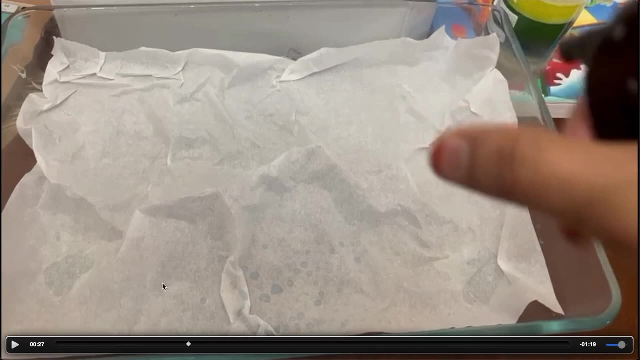 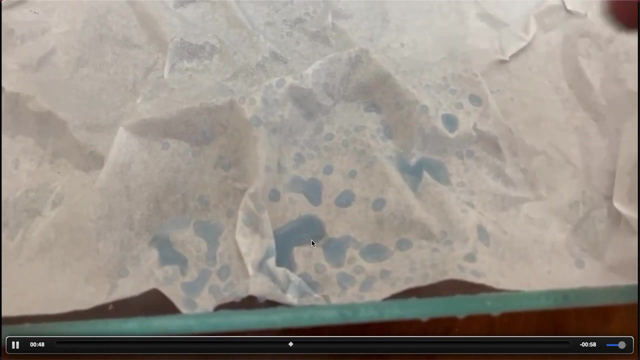 it out on a flat surface and if you can see, in here there's natural formation of places like mountains and ridges and land flat surface. yes, so when you see that the rain falls, all of the water it gets collected in in one spot and most of the water gets streamed. 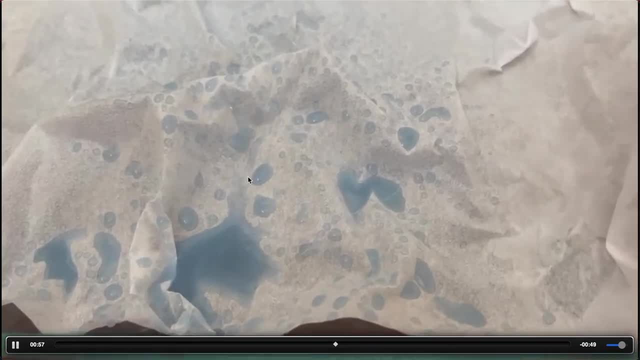 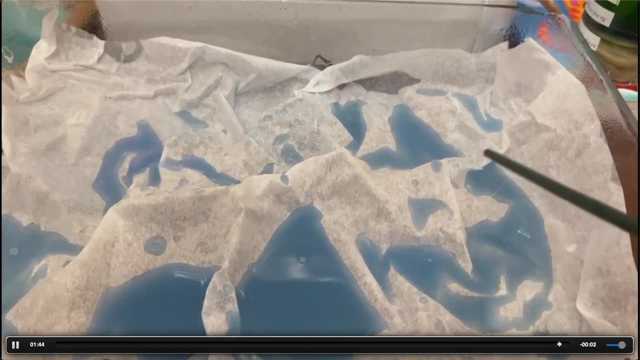 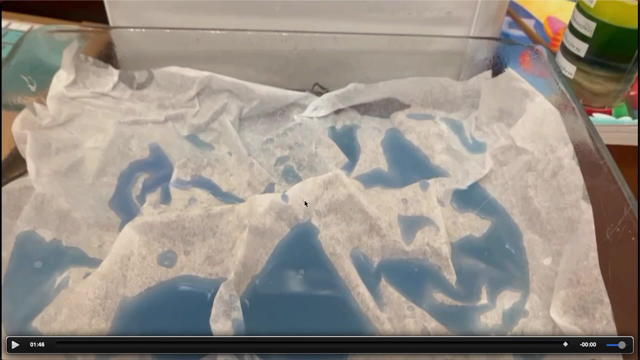 down. yes, if you see in here it's forming a stream to get collected in one place. that would be a lake. these will just keep the water separated. they do not let the water mix. yes, and that would be watershed. so you can see how that anywhere the water falls, it gets drained to one particular spot. 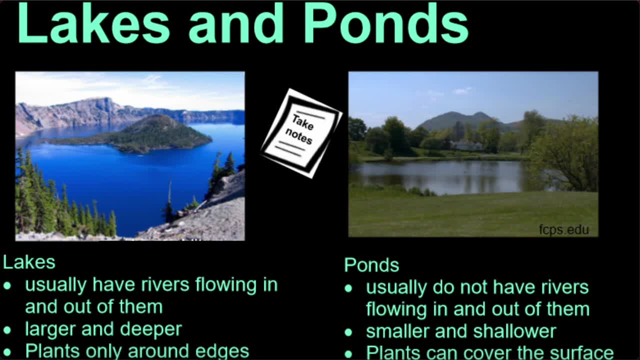 so to the next slide. we know that the surface water water was of three types. yes, the rivers, the lakes and the ponds. so we just saw about river. let's see about lakes and ponds. how is lake different from pond? lakes are usually bigger and ponds are smaller. lakes usually have rivers flowing in and 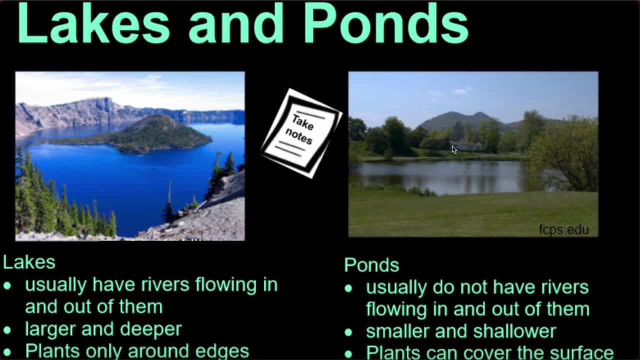 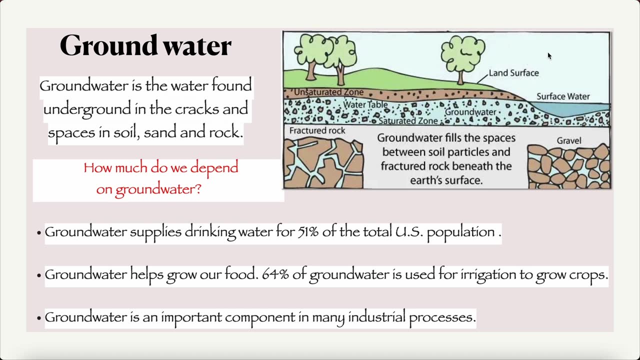 out of them, whereas ponds they are. they don't have rivers flowing in and out of them. plants are around the edges. you can see the plants around the edges, the plants. they cover the surface, sometimes on. next, moving on to the groundwater, where does this groundwater form? so we know that. 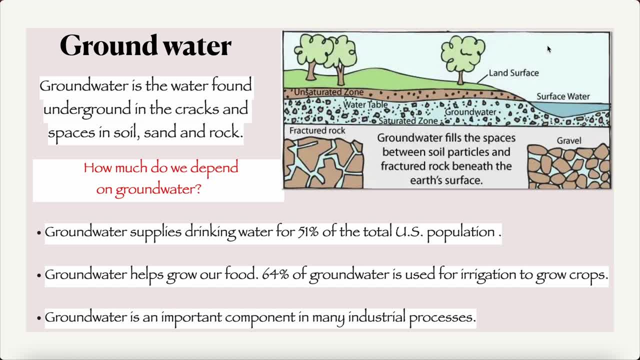 during precipitation, that's during rainfall, all the water falls in the ocean. of the precipitation that falls on the land, most evaporates and some amount of water may run into streams again to the, to the oceans or the seas, but most of it sweeps into the ground and that's what creates the 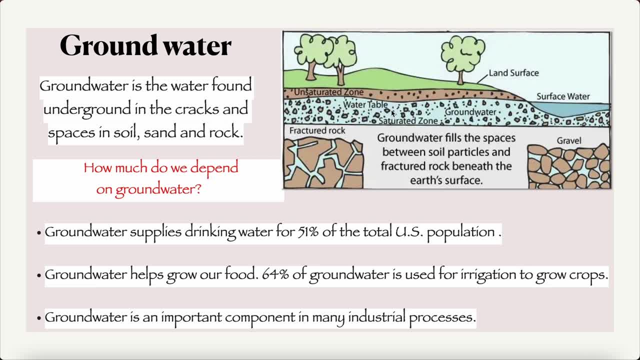 groundwater. groundwater is the water found underground in the cracks and spaces in the soil, sand and rocks. how much do we depend on groundwater? groundwater supplies water for 51 percent of the total united states population. groundwater helps grow over 64 percent of irrigation and irrigation to grow crops. groundwater is an important component. 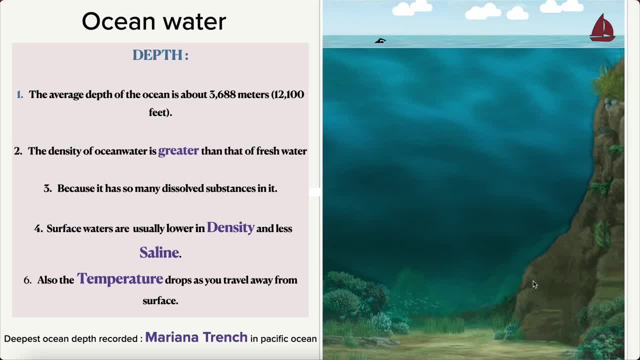 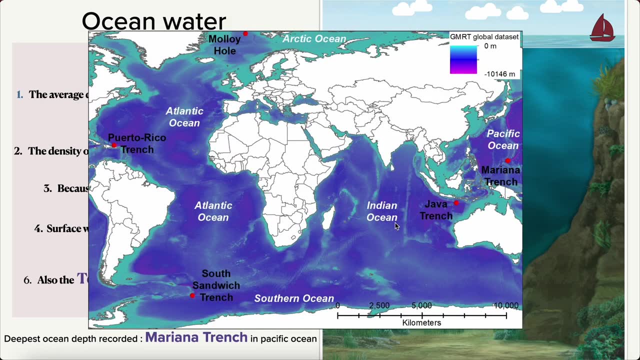 in many industrial processes. next, moving on to the ocean water, that's the salt water. yes, atlantic, indian, pacific and arctic oceans are the names of different parts of ocean. pacific ocean is the largest, covering an area greater than all the land on the earth. seas are generally smaller salt water. 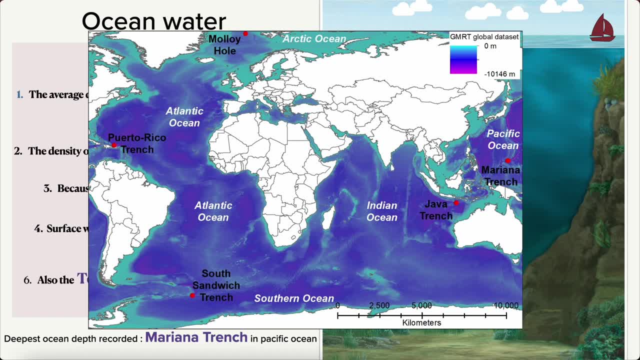 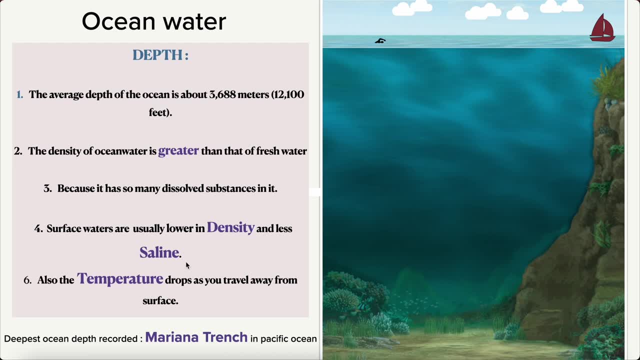 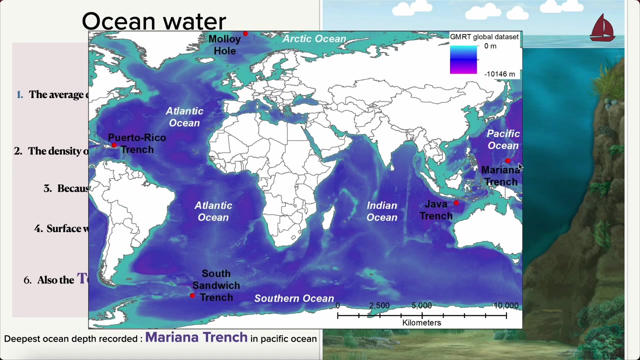 bodies. okay, and what do we know about oceans- water? there are several ways the ocean is unique in the. the water in the earth's ocean varies in salinity, density and temperature. let's see how deep the oceans can be. the average depth of ocean is about 3688 meters. that's the deepest that we have recorded. the density of ocean water is greater than that of the fresh water and the density is high as you go down the ocean surface. water is usually lower in density and less saline. also, the temperature drops as you travel away from the surface of the water. the deepest ocean depth ever recorded is the mariana trench in the pacific ocean. that's over here. 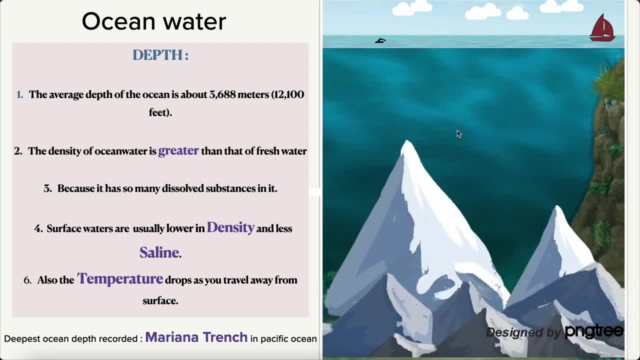 do you know how deep the ocean is? even if you place the mount everest at its bottom, there will be still 6 000 feet left to cover. that's how deep oceans can be. that's what we have recorded. we don't know how deep it is. that could be more. 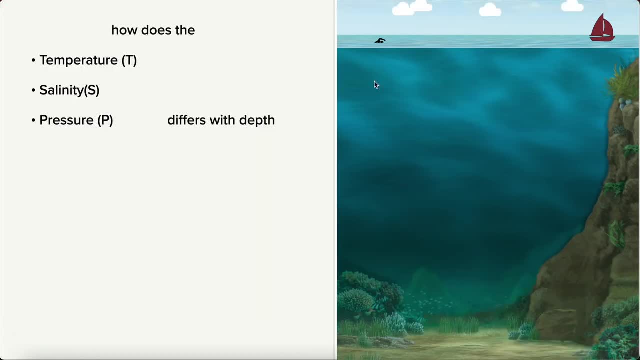 so how is the temperature going to be on the surface of the ocean water? is it going to be high or is it going to be low? it's gonna be high why? why is it high? because it's close to the sun, yes, so most the surface of the water gets heated up by the sun, so the temperature is gonna be high in here. so how's the 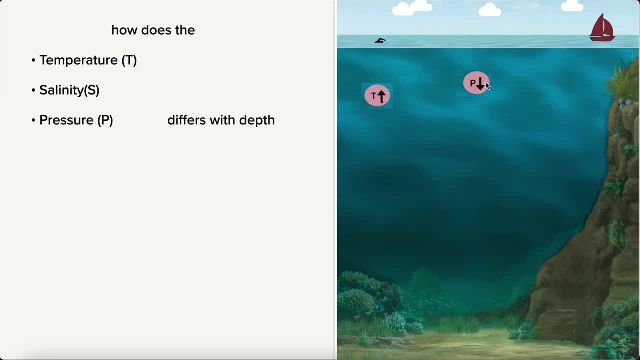 pressure gonna be on the surface of the water? it's gonna be less. why? because it's less dense. the water in here is less then, so there will be less pressure. how is the salinity gonna be in here? it's gonna be less saline. So what about the bottom of the ocean? How is the temperature going to be? It's going to be low. 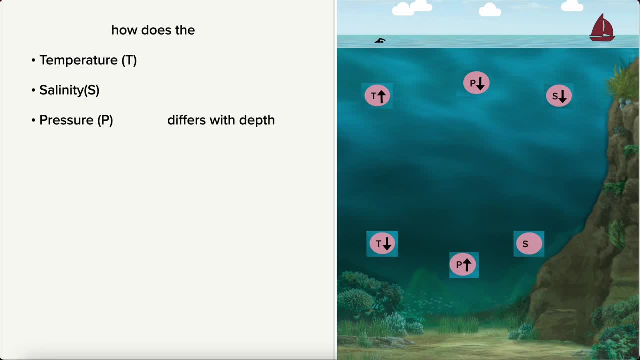 How about the pressure? It's going to be high. How about the salinity? It's going to be high too.